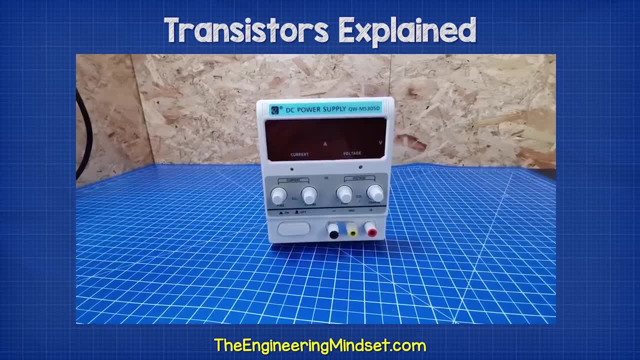 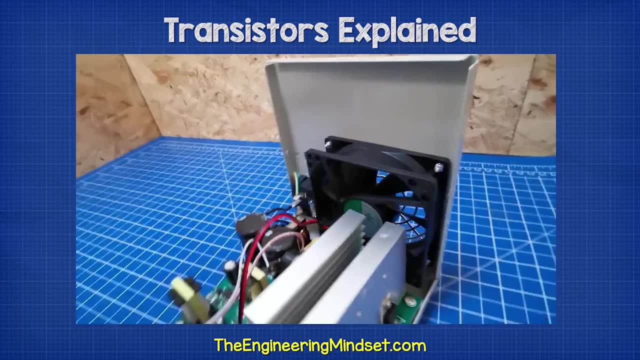 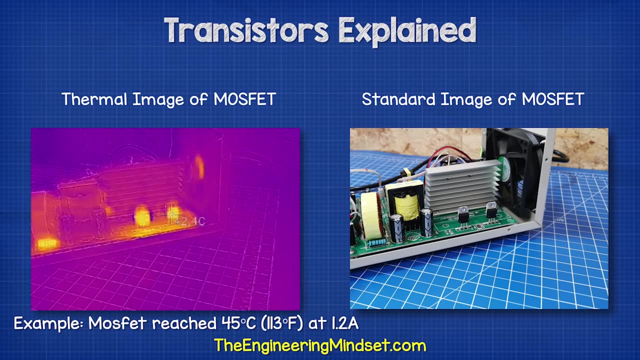 which helps remove the unwanted heat. For example, inside this DC bench power supply we have some MOSFET transistors which are attached to very large heat sinks. Without the heat sink, the components quickly reach 45 degrees celsius or 113 degrees fahrenheit. 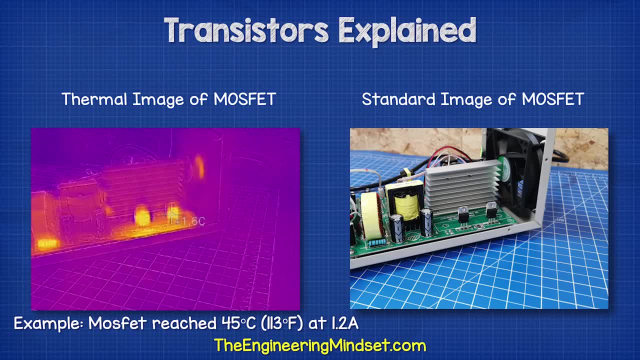 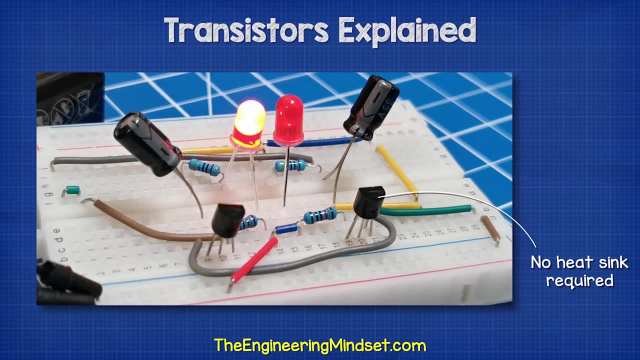 with a current of just 1.2 amps. They will become much hotter as the current increases. but for electronic circuits with small currents we can just use these resin body transistors which do not require a heat sink On the body of the transistor. 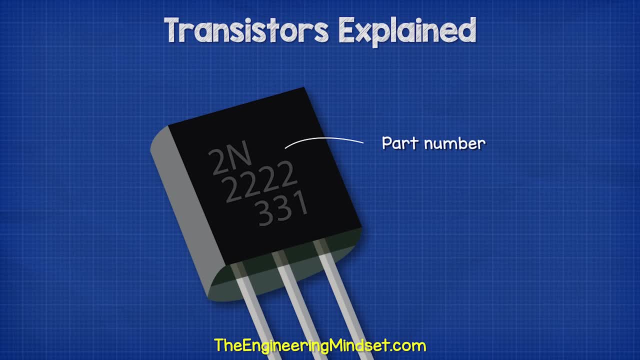 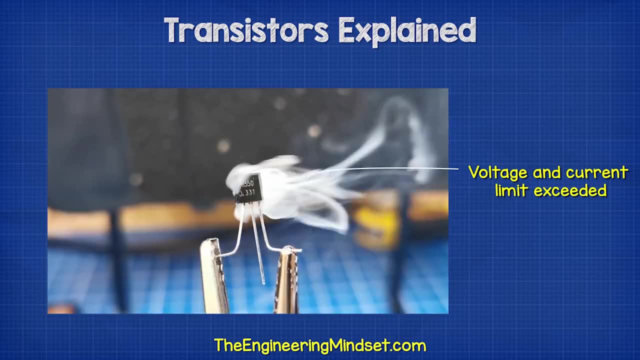 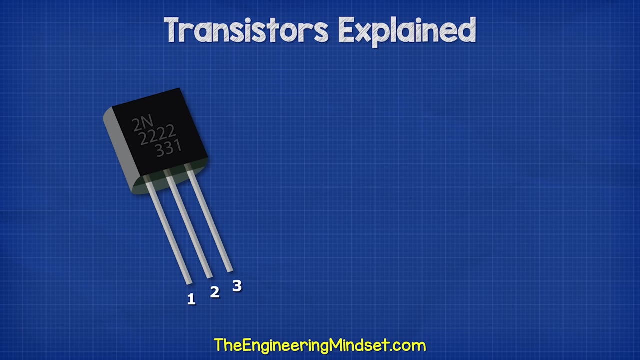 we find some text. This will tell us the part number which we can use to find the manufacturer's data sheet. Each transistor is rated to handle a certain voltage and current, so it's important to check these sheets. Now. with a transistor, we have three pins labeled E, B and C. This stands: 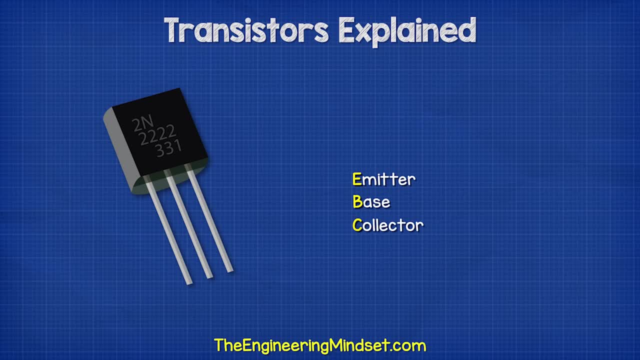 for the emitter and the emitter. The emitter and the emitter are the same. The emitter and the emitter are the base and the collector. Typically with these resin body type transistors with a flat edge, the left pin is the emitter, The middle is the base and the right side is the collector. However, not all. 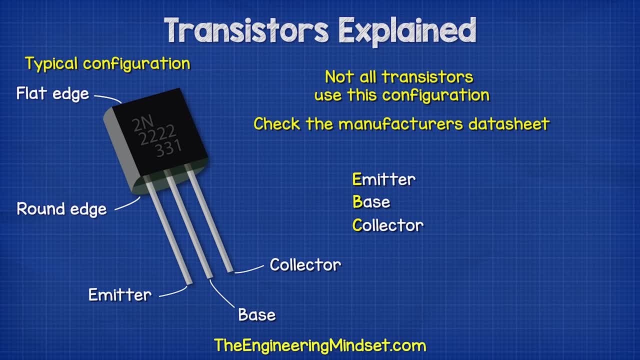 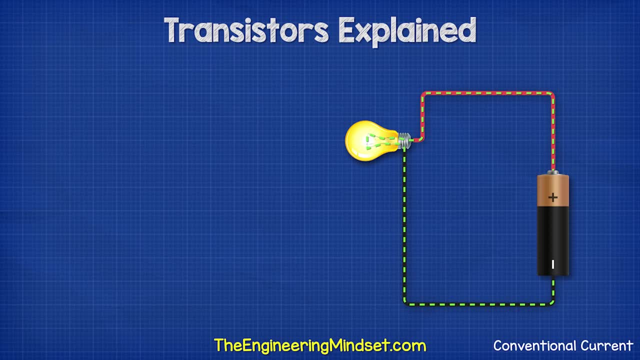 transistors use this configuration, so do check the manufacturer's data sheet. We know that if we connect a light bulb to a battery, it will illuminate. We can install a switch into the circuit and control the light by interrupting the power supply, But this requires a human to manually. 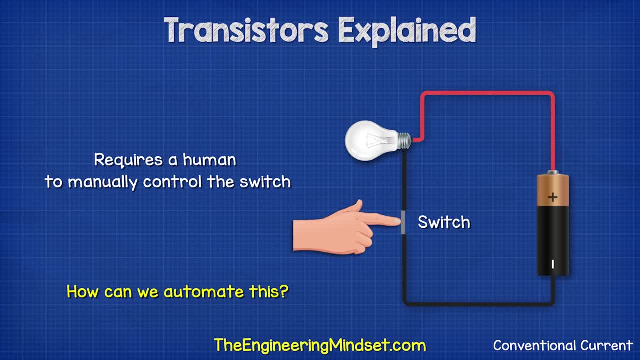 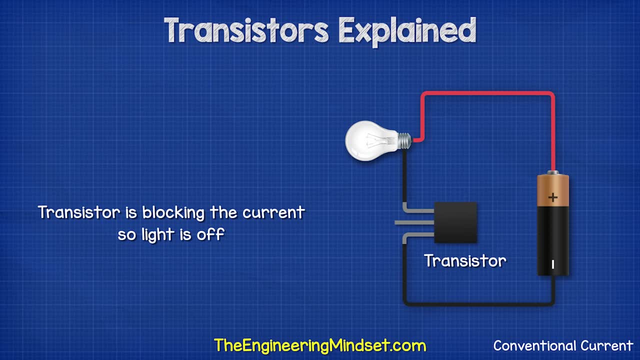 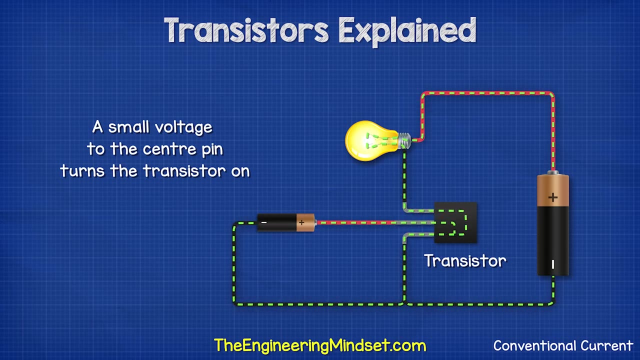 control the switch. So how can we automate this? For that we use a transistor. This transistor is blocking the flow of current, so the light is off. But if we provide a small voltage to the base pin in the middle, it causes the transistor to start allowing current to flow. 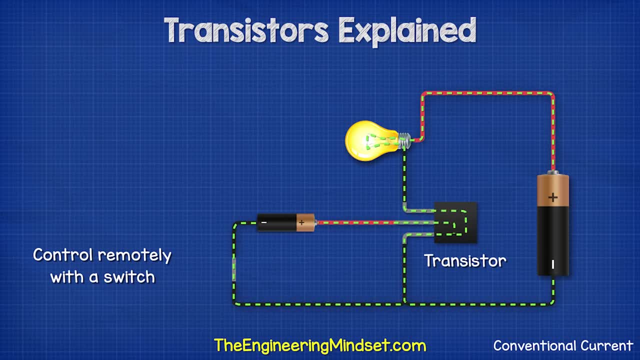 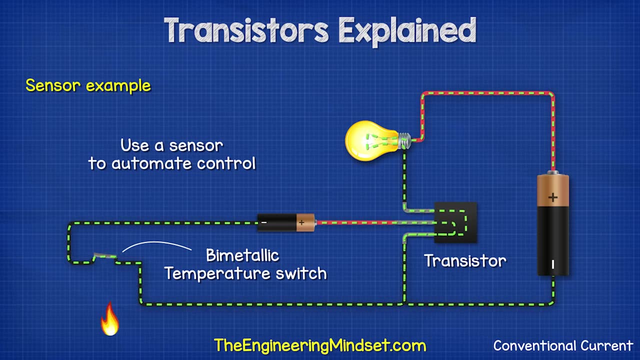 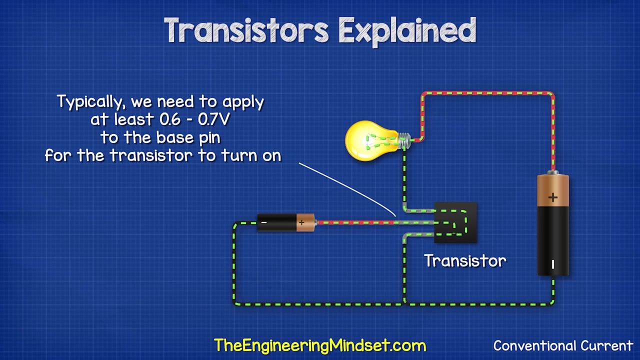 in the main circuit, So the light turns on. We can then place a switch on the controlling to operate it remotely, or we can place a sensor on this to automate the control. Typically, we need to apply at least 0.6 to 0.7 volts to the base pin for the transistor to turn on, For example. 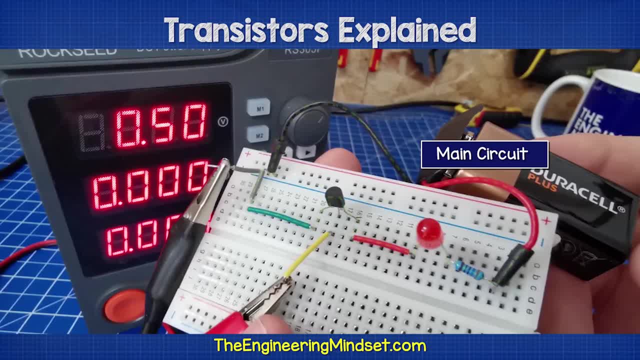 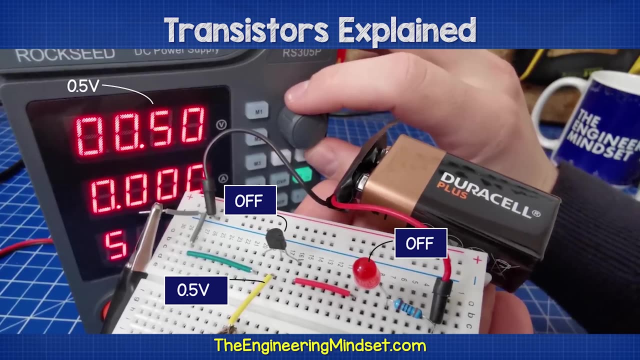 this simple transistor circuit has a red LED and a 9 volt power supply across the main circuit. The base pin is connected to the DC bench power supply. The circuit diagram looks like this: When the supply voltage to the base pin is 0.5 volts, the transistor is off, so the LED is also off. 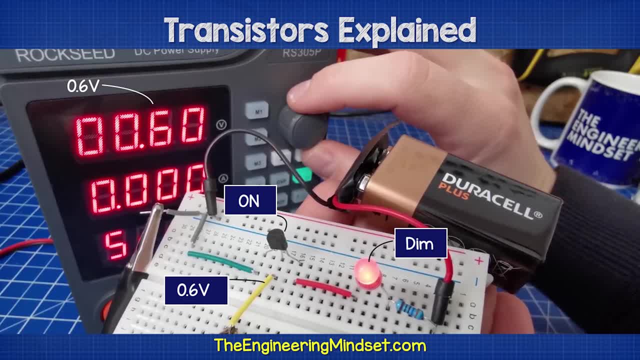 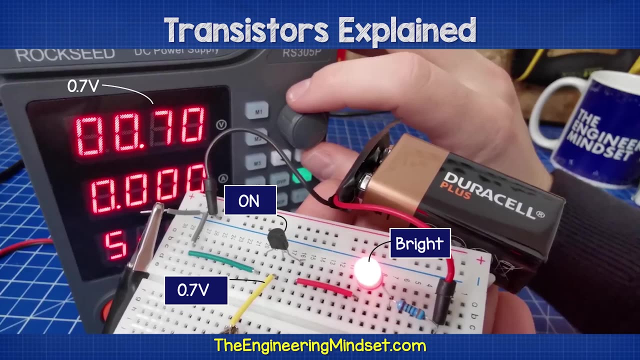 At 0.6 volts, the transistor is on, but not fully. The LED is dim because the transistor is not yet letting the full current flow through the main circuit. Then, at 0.7 volts, the LED is brighter because the transistor is letting almost the full current through. 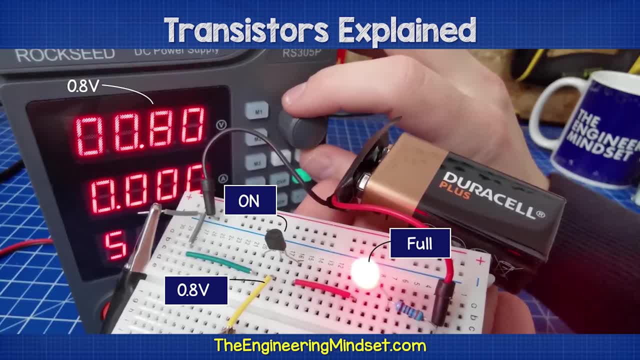 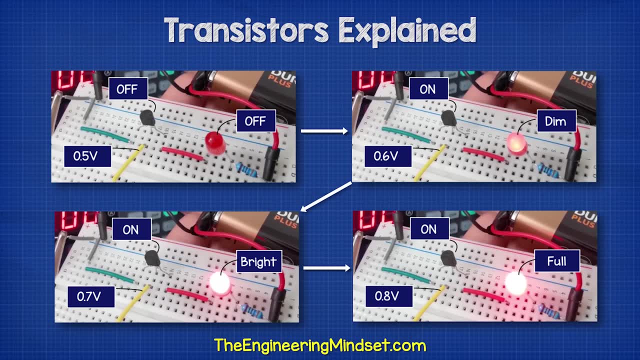 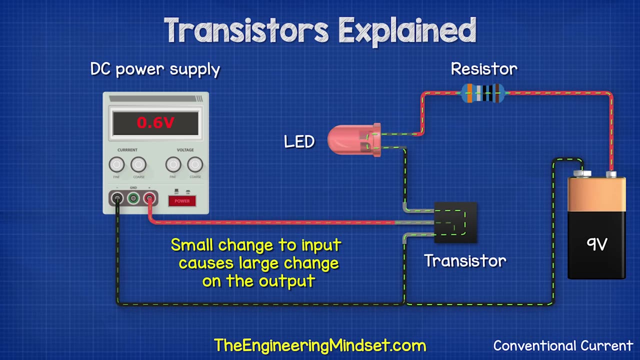 At 0.8 volts. the LED is at full brightness, The transistor is fully open. So what's happening is we're using a small voltage and current to control a larger voltage and current. We saw that a small change to the voltage on the base pin. 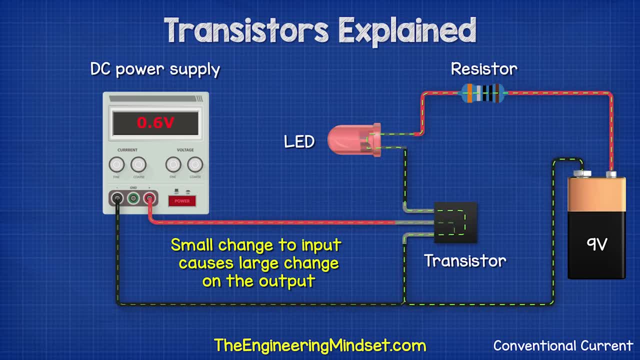 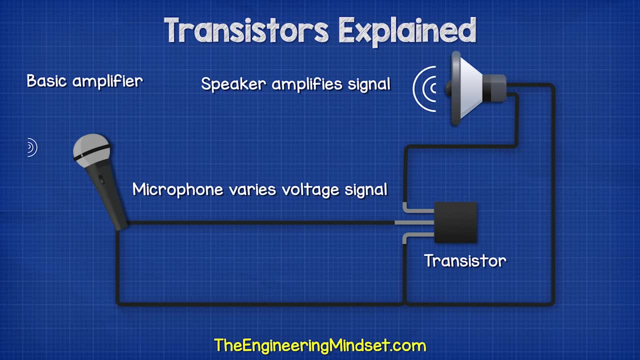 causes a large change on the main circuit. Therefore, if we input a signal to the base pin, the transistor acts as an amplifier. We could connect a microphone which varies the voltage signal on the base pin and this will amplify a speaker in the main circuit to form a very 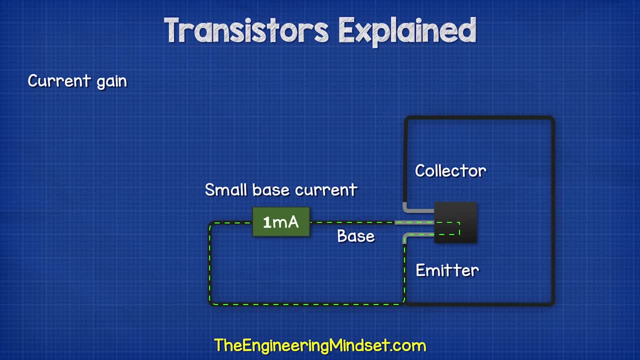 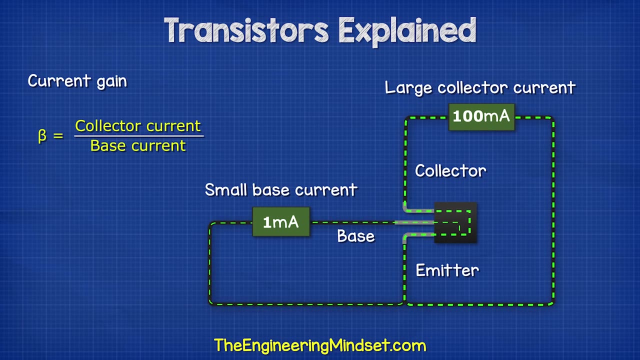 basic amplifier. Typically there is a very small current on the base pin, perhaps just 1 milliamps or even less. The collector has a much higher current, for example 100 milliamps. The ratio between these two is known as the current gain and uses the symbol beta. We can find the ratio. 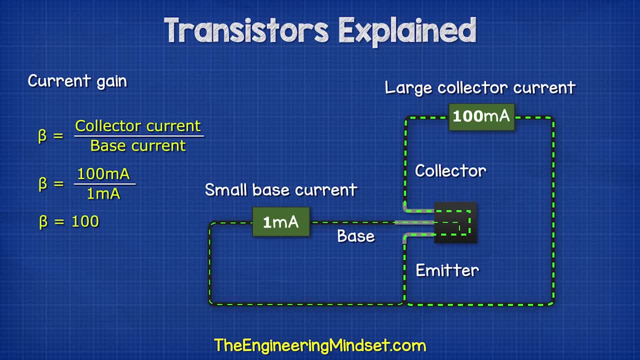 in the manufacturer's datasheet. In this example we can find the current gain in the manufacturer's data sheet. For example, the collector current is 100 milliamps and the base current is 1 milliamp. so the ratio is 100 divided by 1, which gives us 100.. We can also rearrange this formula to find the currents also. 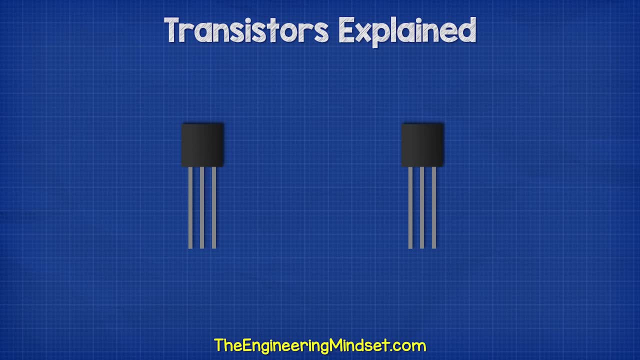 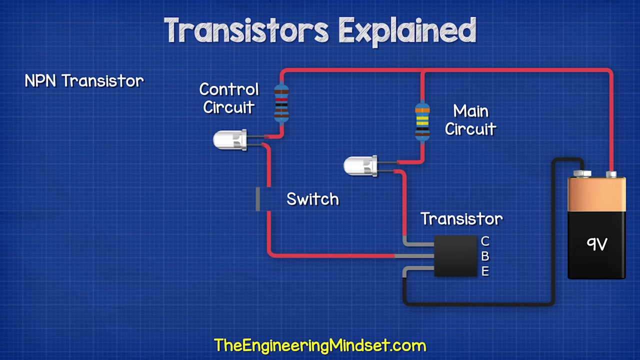 We have two main types of bipolar transistors: the NPN and the PNP type. The two transistors look nearly identical so we need to check the part number to tell which is which. With an NPN transistor we have the main circuit and the control circuit. 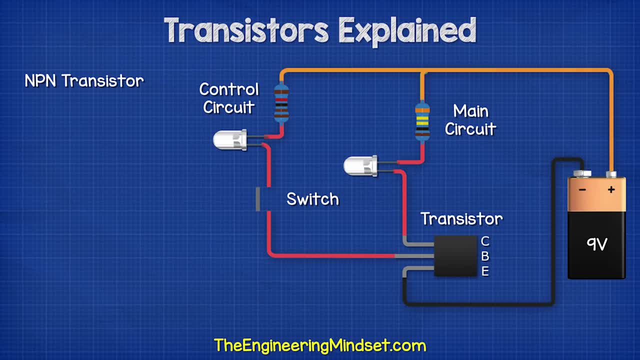 Both are connected to the positive of the battery. The main circuit is off until we press the switch on the control circuit. We can see the current is flowing through both wires to the transistor. We can remove the main circuit and the control circuit led will still turn on when the switch. 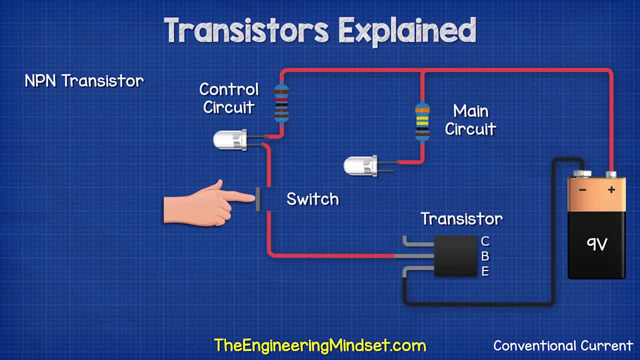 is pressed, as the current is returning to the battery through the transistor. In this simplified example, when the switch is pressed, there are 5 milliamps flowing into the base pin, there are 20 milliamps flowing into the collector pin and 25 milliamps flowing 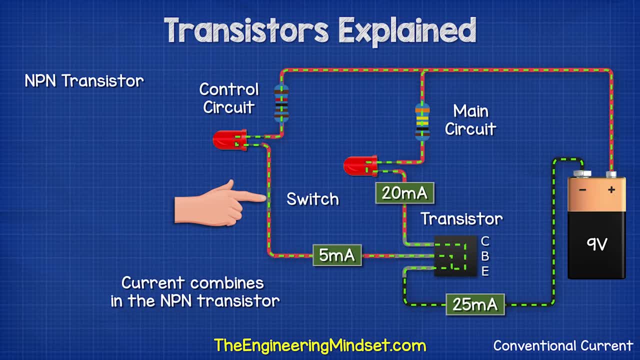 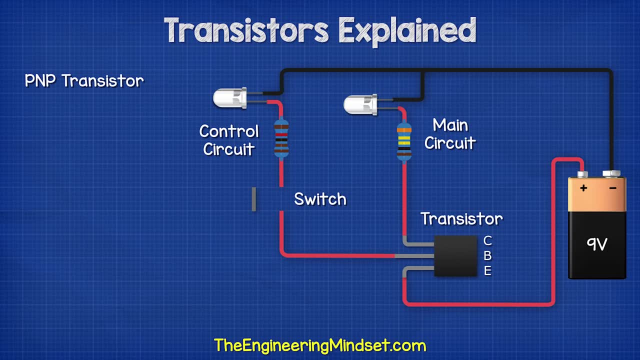 out of the emitter. The current therefore combines in this transistor With a PNP transistor. we again have the main circuit and the control circuit, but now the emitter is connected to the positive of the battery. The main circuit is off until we press the switch. We can see the current is still on until we press the switch. 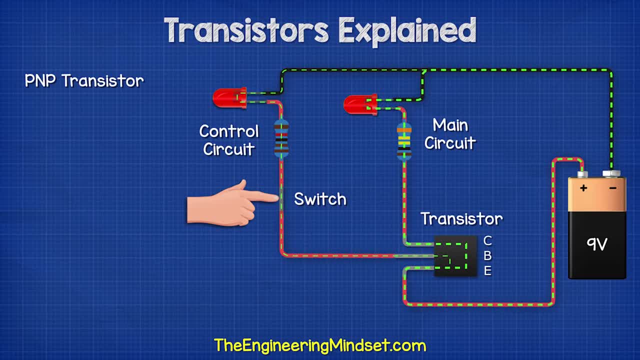 until we press the switch on the control circuit. We can see with this type that some of the current flows out of the base pin and returns to the battery. The rest of the current flows through the transistor and through the main LED and then back to the battery. 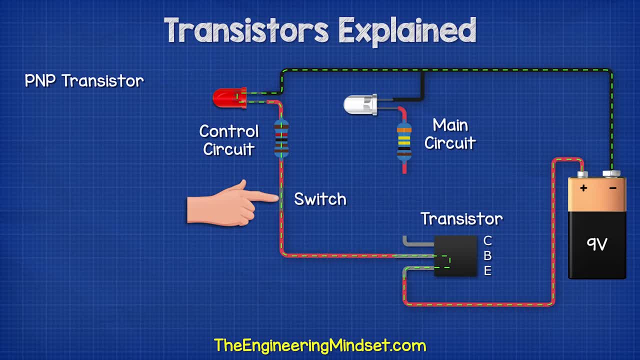 If we remove the main circuit, the control circuit LED will still turn on. In this example, when the switch is pressed, there are 25 milliamps flowing into the emitter, 20 milliamps flowing out of the collector and five milliamps flowing out of the base. 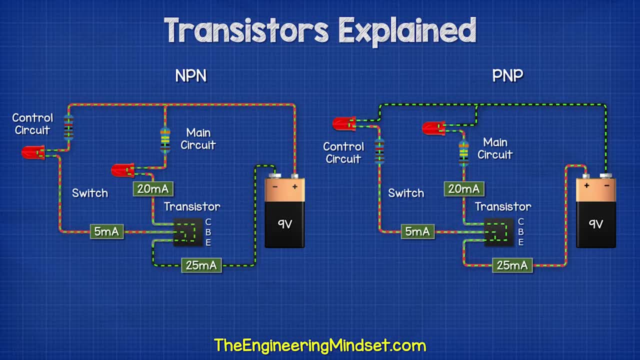 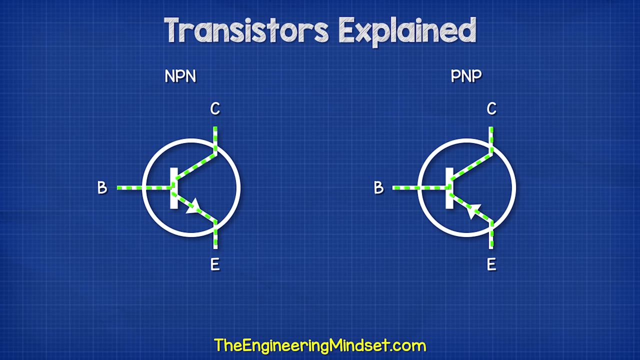 The current therefore divides in this transistor. I'll place these side by side so you can see how they compare. Transistors are shown on electrical drawings with symbols like these. The arrow is placed on the emitter. The arrow points in the direction of conventional current. 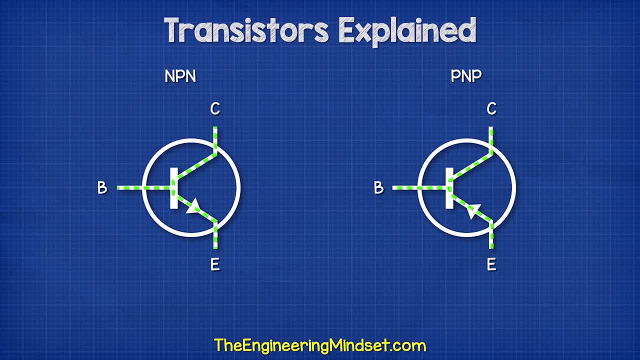 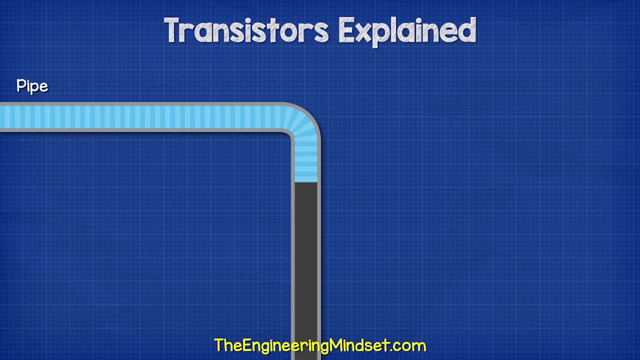 so that we know how to connect them into our circuits. To understand how a transistor works, I want you to first imagine water flowing through a pipe. It flows freely through the pipe until we block it with a disc. Now, if we connect a smaller pipe into the main one, 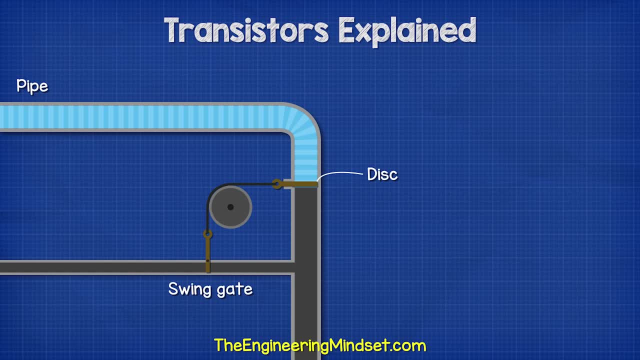 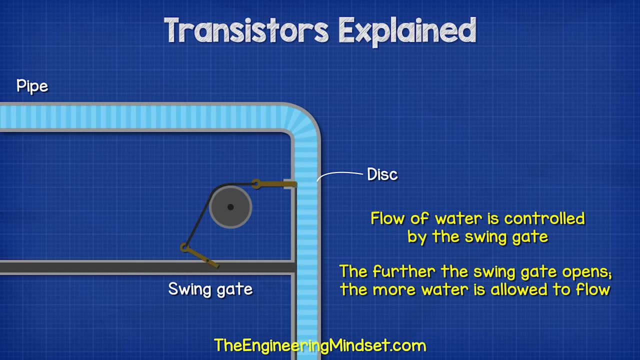 and place a swing gate within this small pipe. we can move the disc using a pulley. The further the swing gate opens, the more water is allowed to flow in the main pipe. The swing gate is a little heavy, so a small amount of water is allowed to flow in the main pipe. The swing gate is a little heavy. 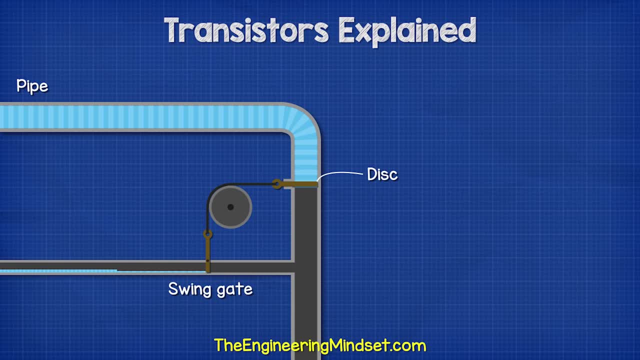 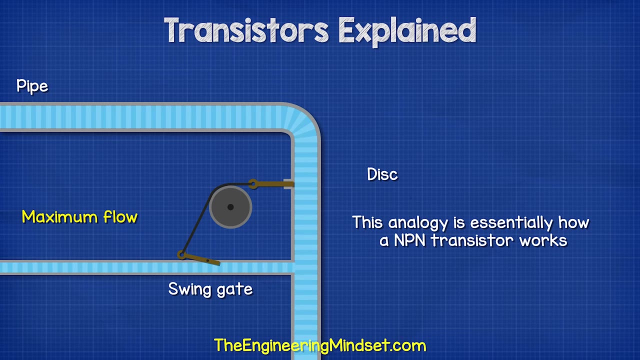 so a small amount of water is allowed to flow in the main pipe. A certain amount of water is required to force the gate to open. The more water we have flowing in this small pipe, the further the valve opens and allows more and more water to flow in the main pipe. 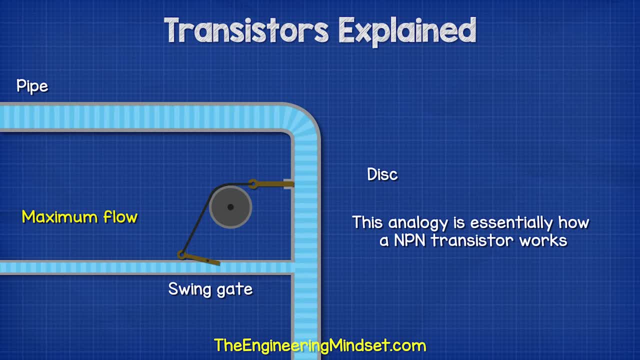 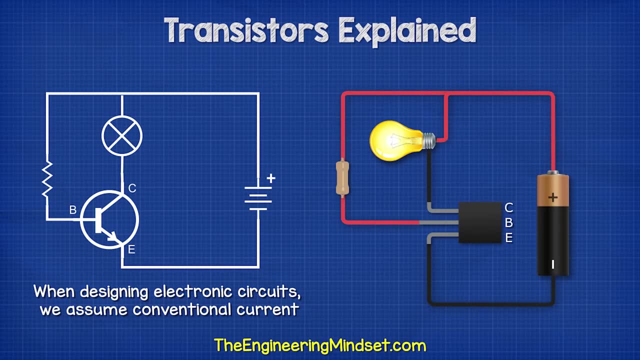 This is essentially how an NPN transistor works. You might already know that when we design electronic circuits we use conventional current. So in this NPN transistor circuit We assume that the current is flowing from the battery's positive into both the collector and the base pin and then out of the emitter pin. 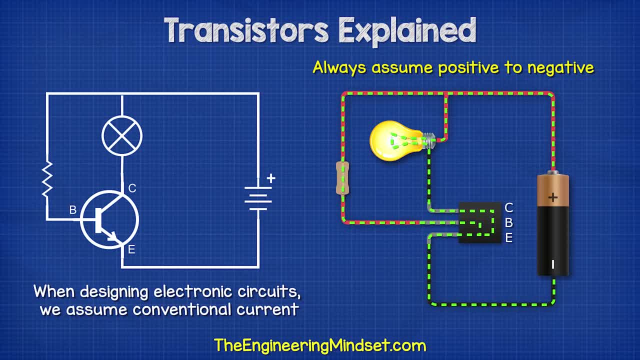 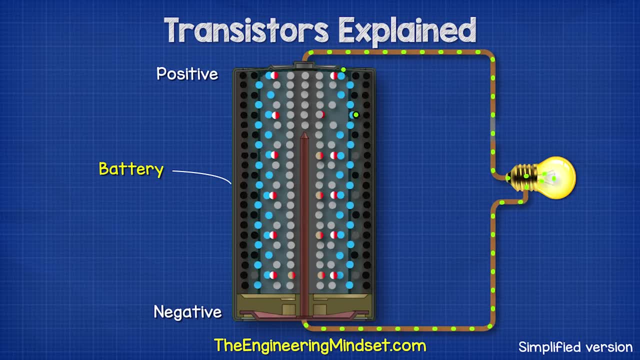 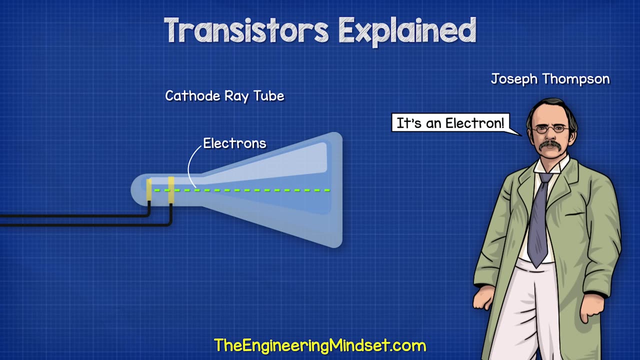 We always use this direction to design our circuits. However, that's not what's actually occurring In reality. the electrons are flowing from the negative to the positive of the battery. This was proved by Joseph Thompson, who carried out some experiments to discover the electron. 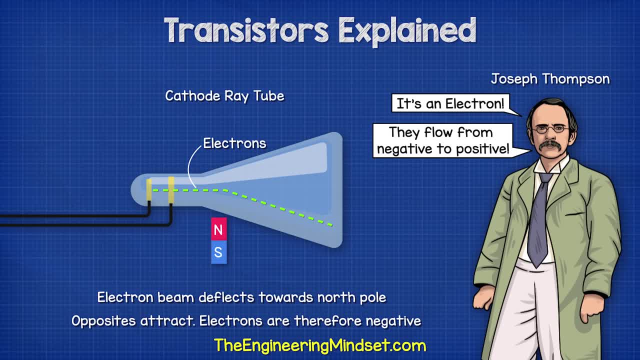 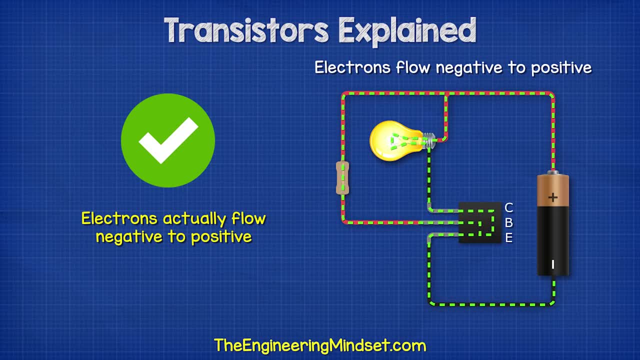 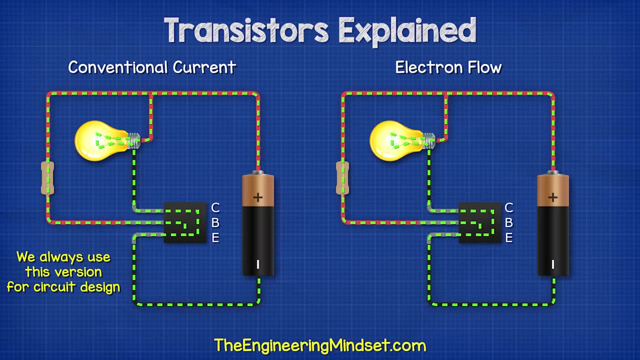 and also prove they flowed in the opposite direction. So in reality electrons flow from the negative into the emitter and then out of the collector and the base pin. We call this electron flow. I'll place these side by side so you can see the difference in the two theories. 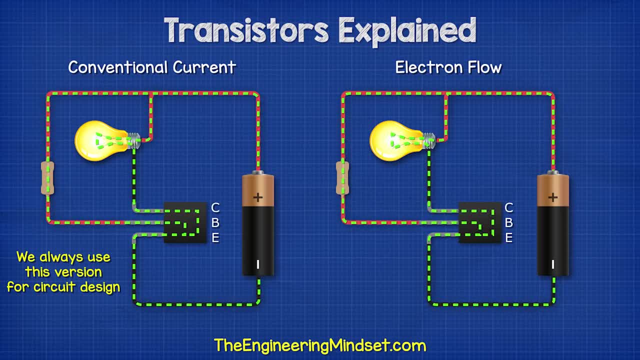 Remember, we always design circuits using the conventional current method, But scientists and engineers know that electron flow is how it actually works. So let's look at how electron flow works. By the way, we have also covered how a battery works in detail in our previous video. 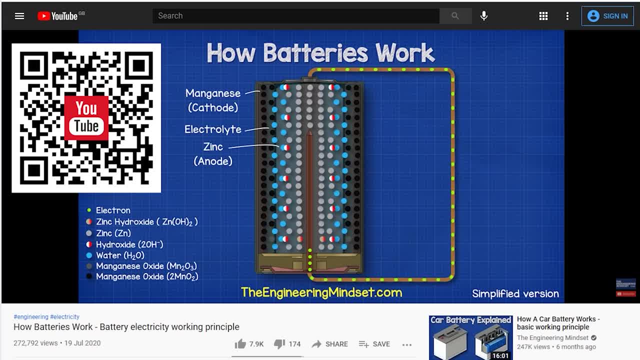 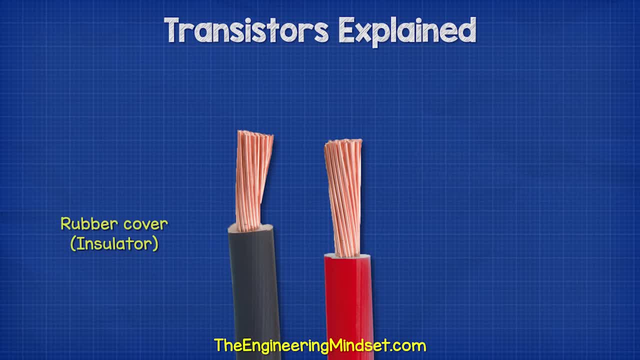 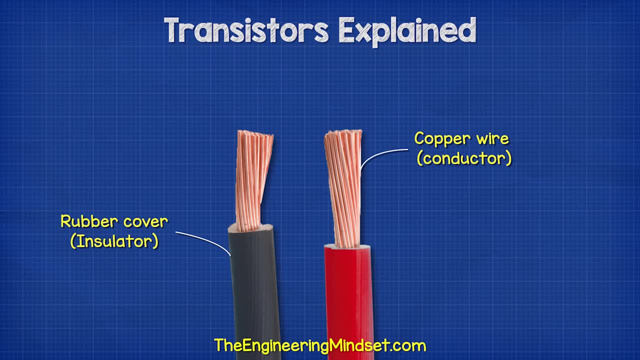 Do check that out. Links can be found in the video description down below. OK, so we know that electricity is the flow of electrons through a wire. The copper wire is the conductor and the rubber is the insulator. Electrons can flow easily through the copper, but they can't flow through the rubber insulator. 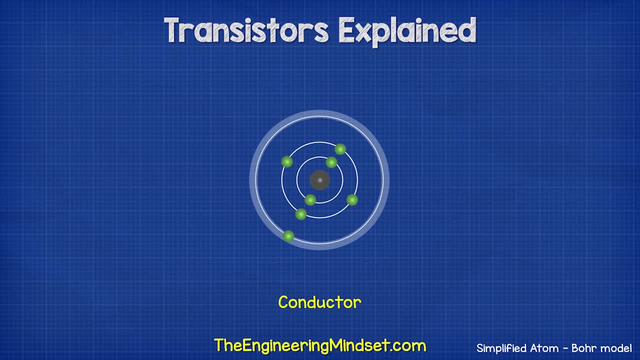 If we look at this basic model of an atom, of a metal conductor, we have the nucleus at the center And this is surrounded by a number of orbital shells which hold the electrons. Each shell holds a maximum number of electrons And an electron needs to have a certain amount of energy to be accepted into each shell. 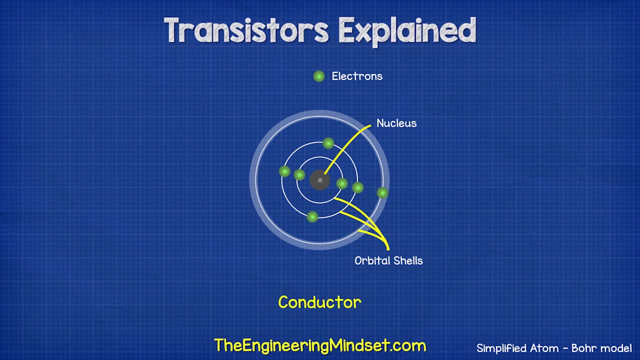 The electrons located furthest away from the nucleus hold the most energy. The outermost shell is known as the valence shell. A conductor has between one and three electrons in its valence shell. The electrons are held in place by the nucleus, But there is another shell known as the conduction band. 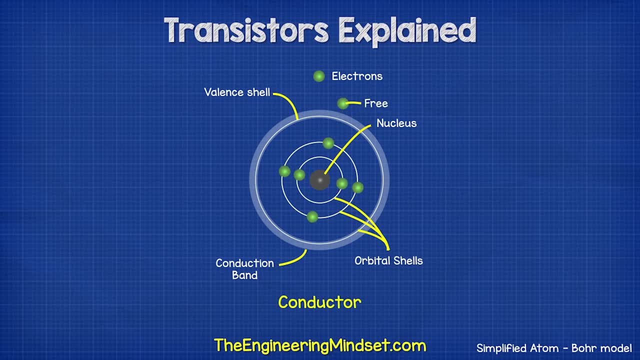 If an electron can reach this, then it can break free from the atom and move to other atoms. With a metal atom, such as copper, the valence shell and the conduction band overlap, So it's very easy for the electrons to move. 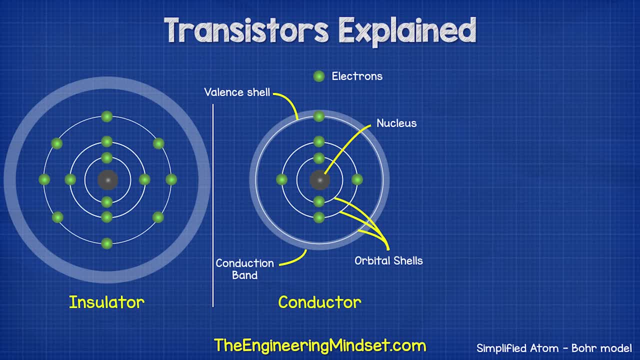 With an insulator. the outermost shell is packed. There's very little to no room for an electron to join. The nucleus has a tight grip on the electrons and the conduction band is far away, So the electrons can't reach this to escape. 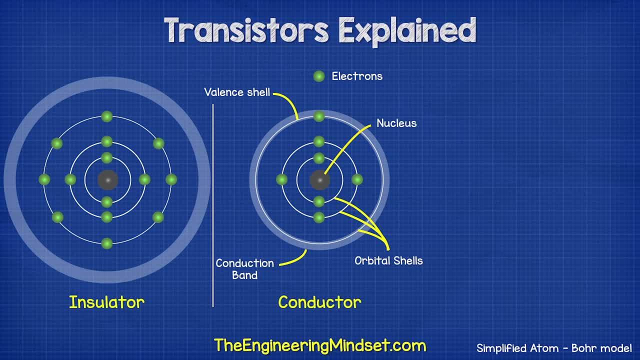 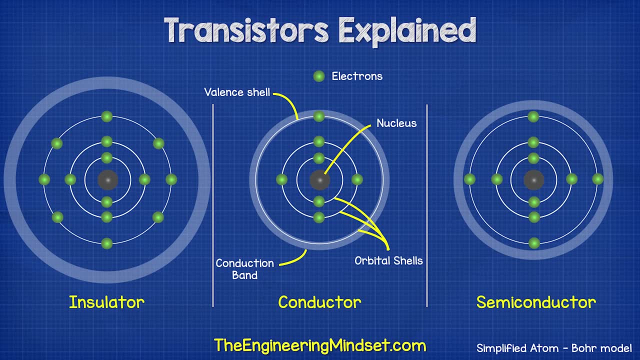 Therefore, electricity cannot flow through this material. However, there's another material known as a semiconductor. Silicon is an example of a semiconductor. With this material, there's one too many electrons in the valence shell for it to be a conductor, So it acts as an insulator. 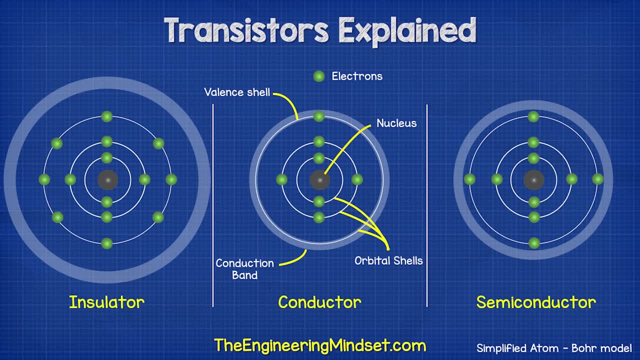 But it's not. But as the conduction band is quite close, if we provide some external energy, some electrons will gain enough energy to make the jump into the conduction band and become free. Therefore, this material can act as both an insulator and a conductor. 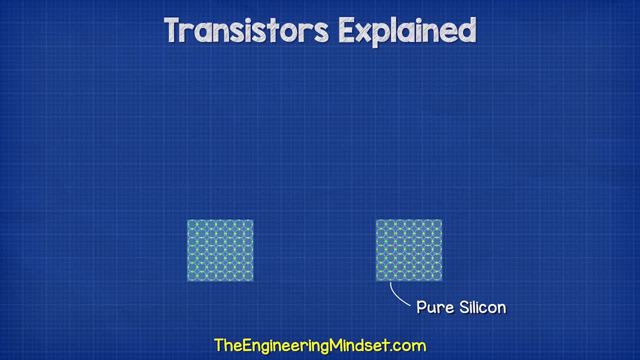 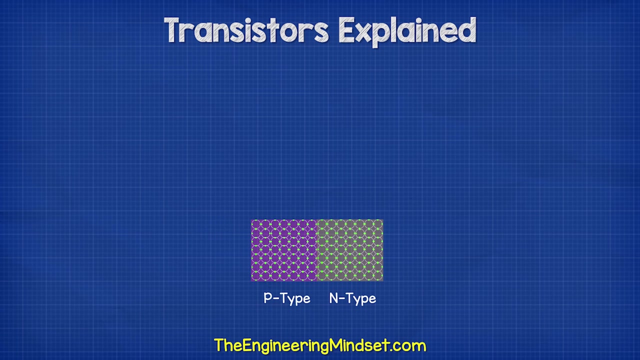 Pure silicon has almost no free electrons. So what engineers do is dope the silicon with a small amount of another material which changes its electrical properties. We call this p-type and n-type doping. We combine these materials to form the p-n junction. 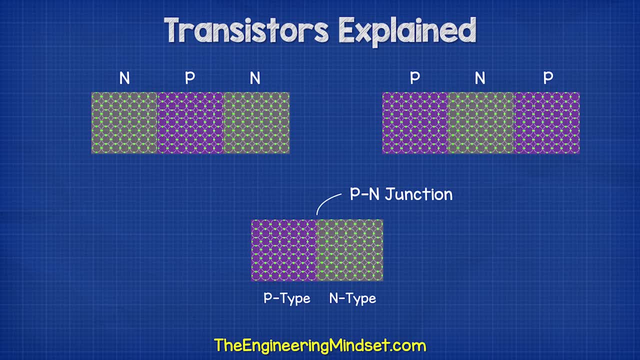 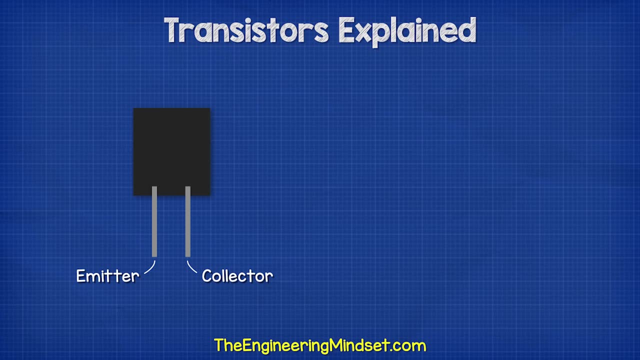 We can sandwich these together to form an n-p-n or a p-n-p transistor. Inside the transistor we have the collector pin and the emitter pin Between these. in an n-p-n transistor we have two layers of n-type material and one layer. 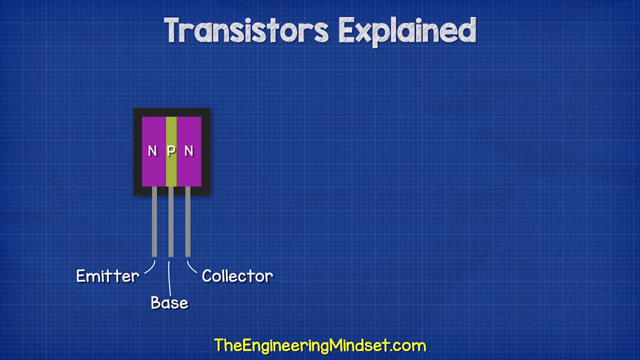 of p-type. The base wire is connected to the p-type layer. The base wire is connected to the p-type layer In a p-n-p transistor. this is just configured the opposite way. The entire thing is enclosed in a resin to protect the internal materials. 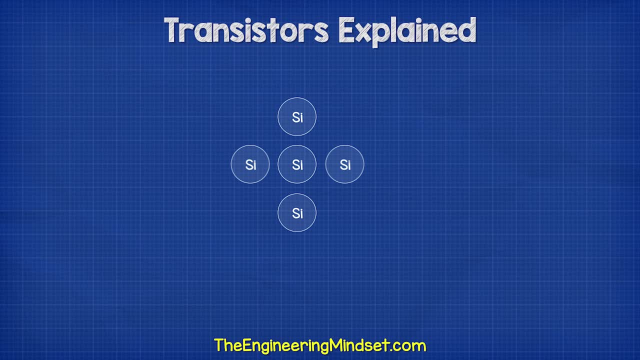 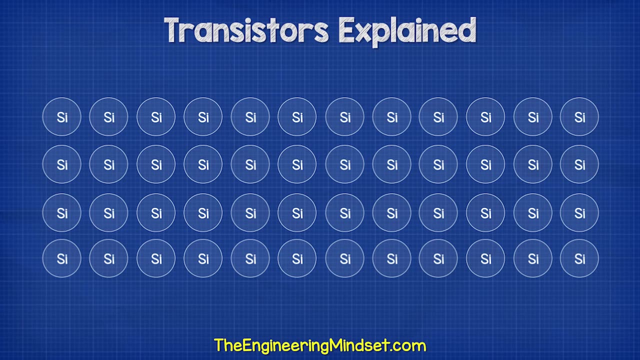 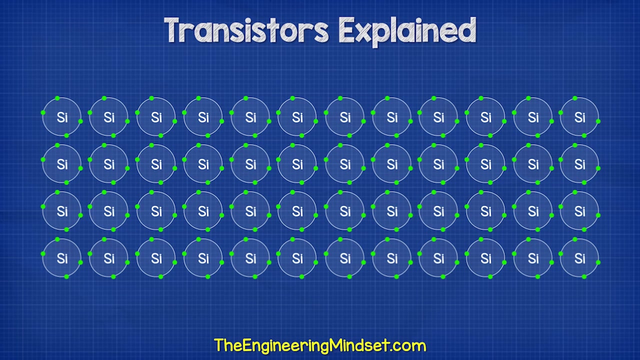 Let's imagine the silicon hasn't been doped yet, so it's just pure silicon. inside Each silicon atom is surrounded by four other silicon atoms. Each atom wants eight electrons in its valence shell, But the silicon atoms only have four electrons in their valence shell, so they sneakily 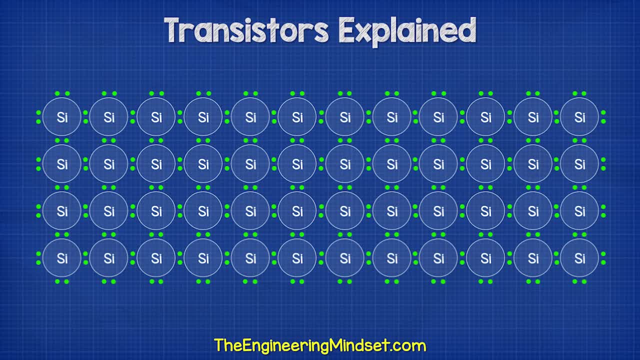 share an electron with their neighboring atom to get the eight they desire. This is known as covalent bonding. When we add the n-type material, such as phosphorus, it will take the position of some of the silicon atoms. The phosphorus atoms have five electrons in their valence shell. 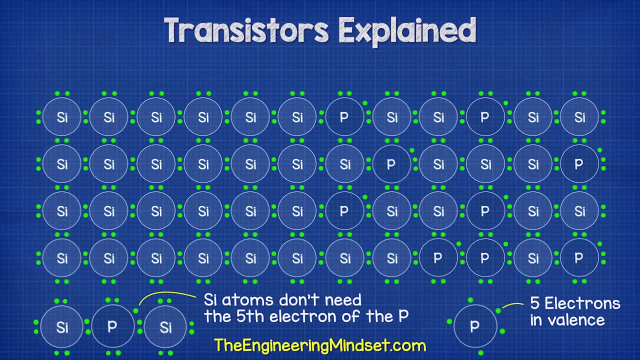 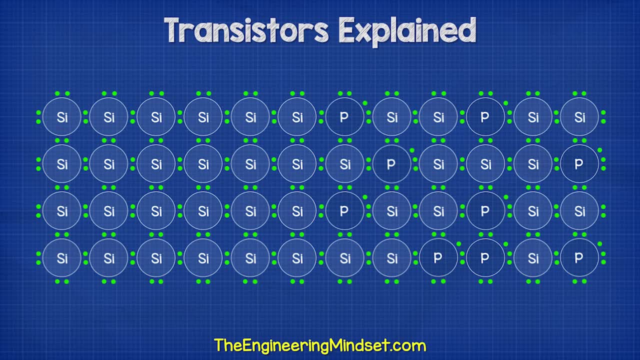 So as the silicon atoms are sharing electrons to get their desired eight, they don't need this extra one, Which means there's now extra electrons in the material And these are free to move around With p-type doping we add in a material such as aluminium or aluminum. 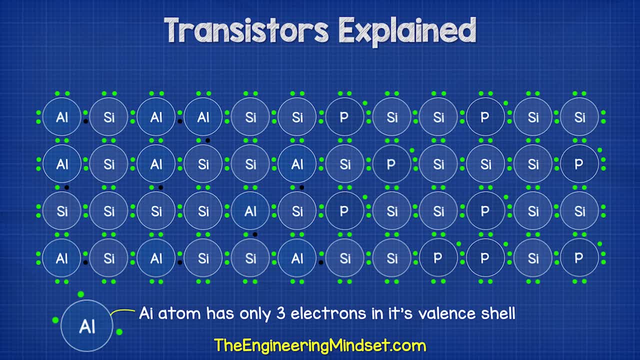 This atom has only three electrons in its valence shell. It therefore can't provide its four neighbors with an electron to share, So one of them will have to go without. This means a hole has been created where an electron can sit and occupy. 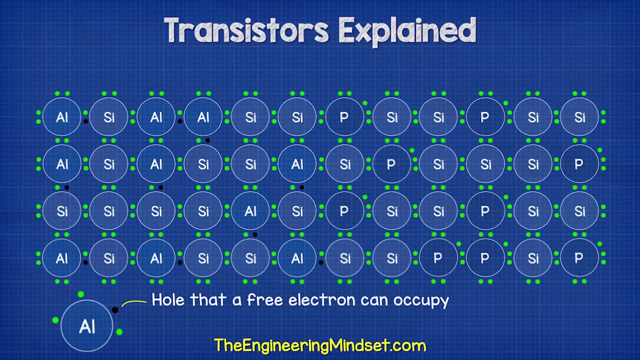 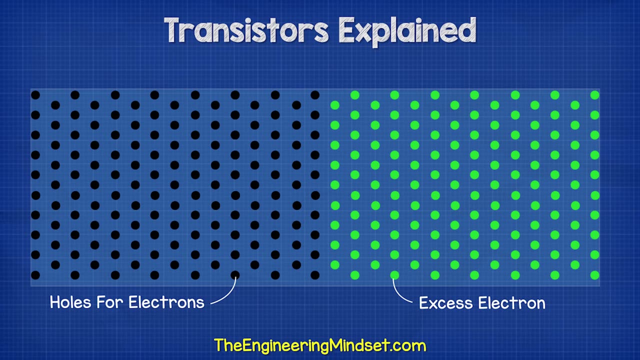 We now have two doped pieces of silicon, One with too many electrons and one with not enough electrons. The two materials join to form a p-n junction. At this junction we get what's known as a depletion region. In this region, some of the excess electrons from the n-side will move over to occupy the 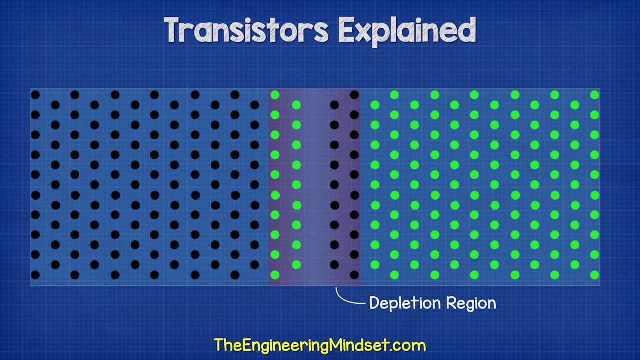 holes in the p-side. This migration will form a barrier, with a buildup of electrons and holes. on opposite sides. The electrons are negatively charged And the holes are therefore considered positively charged, So this buildup causes a slightly negatively charged region and a slightly positively. 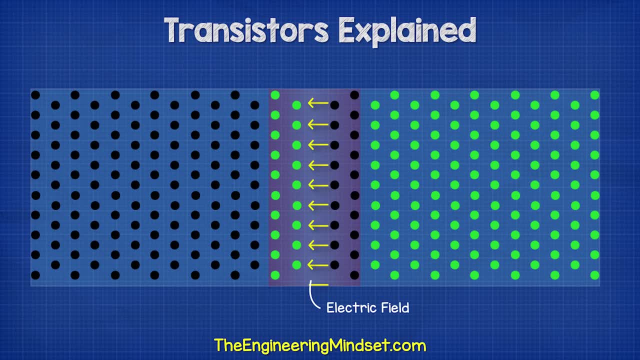 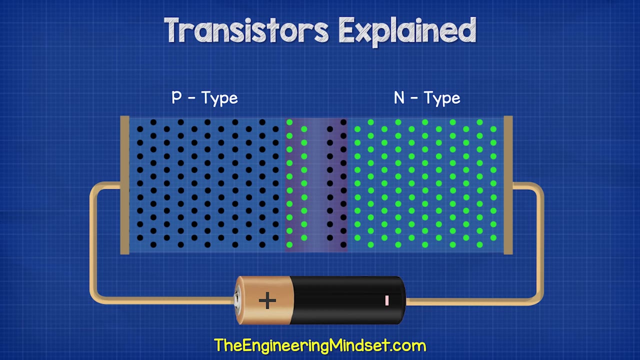 charged region. This creates an electric field and prevents more electrons from moving across. The potential difference across this region is typically around 0.7 volts When we connect a voltage source across the two ends, with the positive connected to the p-type material. 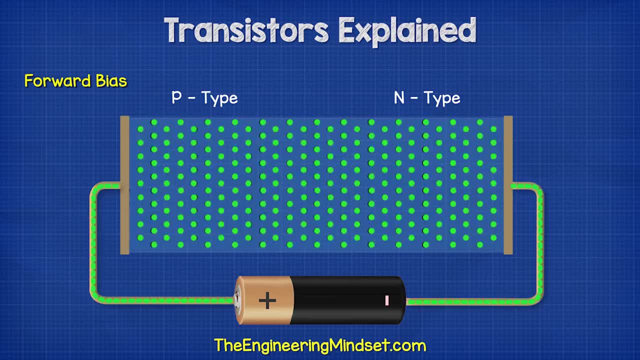 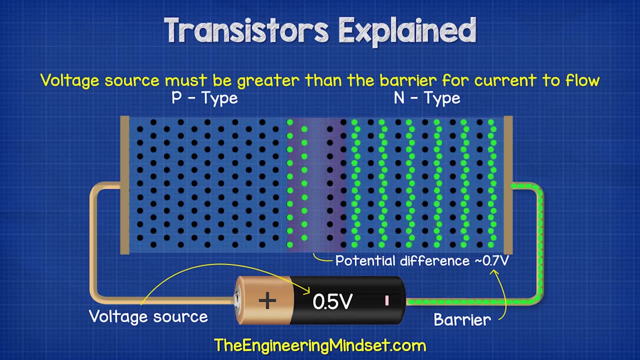 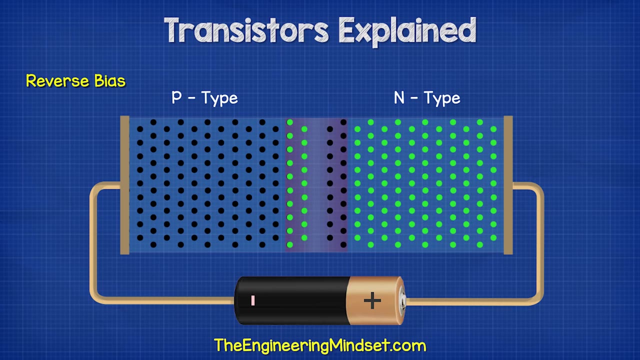 This will create a forward bias and the electrons will begin to flow. The voltage source has to be greater than the 0.7 volt barrier, Otherwise electrons cannot make the jump. When we reverse the power supply so that the positive is connected to the n-type material, 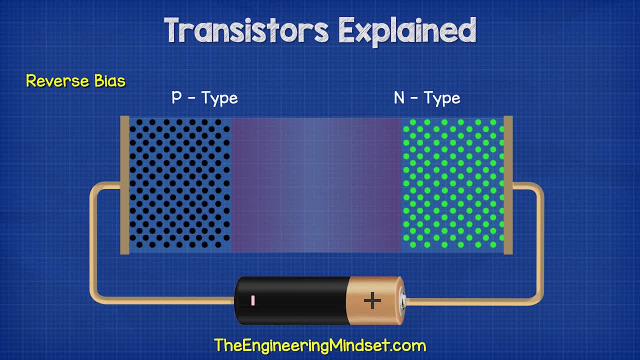 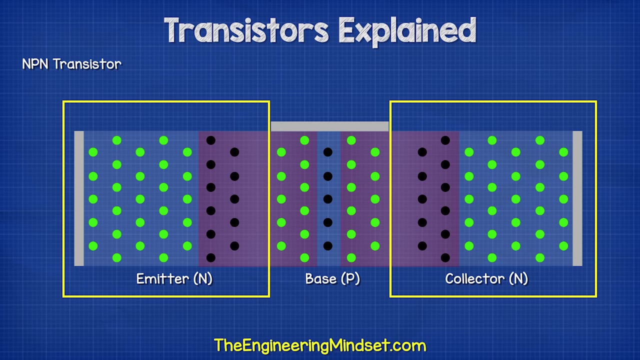 the electrons held in the barrier will be pulled back towards the positive terminal and the holes will be pulled back towards the negative terminal. This has caused a reverse bias In a NPN transistor. we have two layers of n-type material, So we have two junctions and therefore two barriers. 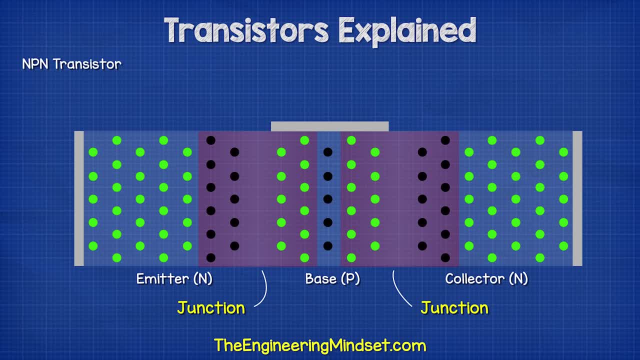 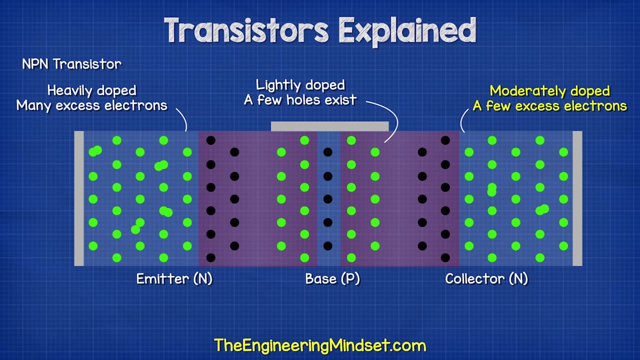 So no current can flow through it. ordinarily The emitter n-type material is heavily doped, So there are a lot of excess electrons here. The base p-type is lightly doped, So there are a few holes here. The collector n-type is moderately doped. 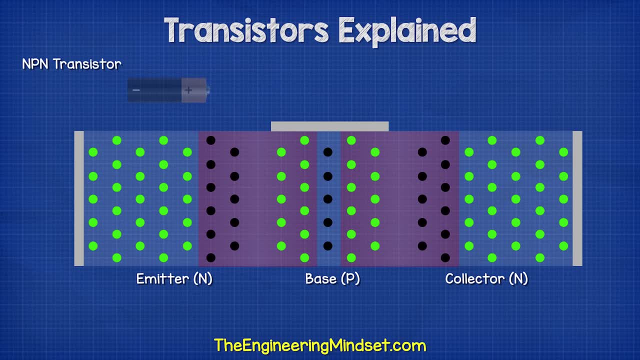 So there are a few holes here, There are a few excess electrons here. If we connect a battery across the base and the emitter with the positive connected to the p-type layer, this will create a forward bias. The forward bias causes the barrier to collapse. 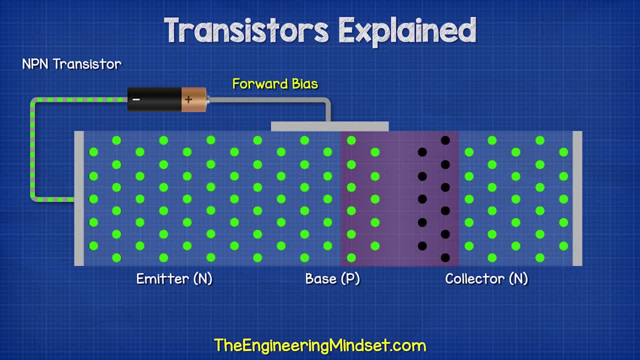 as long as the voltage is at least 0.7 volts. So the barrier diminishes and the electrons rush across to fill the space within the p-type material. Some of these electrons will occupy a hole and they will be pulled towards the positive terminal of the battery. 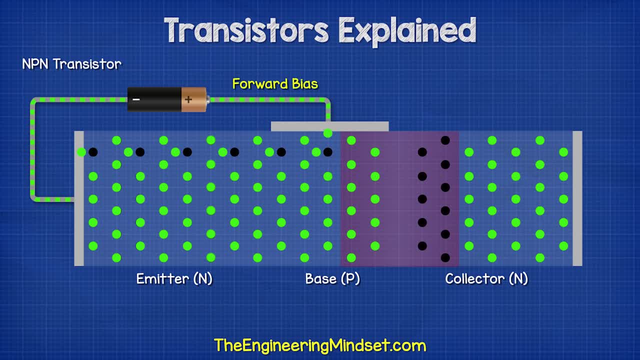 The p-type layer is thin and was lightly doped on purpose so that there is a low chance of electrons falling into a hole. The rest will remain free to move around the material. Therefore, only a small current will flow out of the base pin. 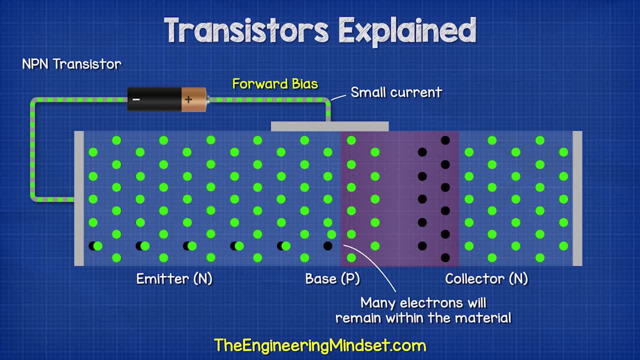 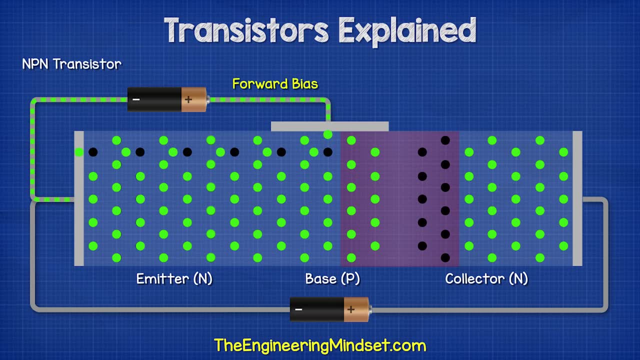 leaving an excess of electrons now in the p-type material. If we then connect another battery between the emitter and the collector, with the positive connected to the collector, the negatively charged electrons within the collector will be drawn to the positive terminal, which causes a reverse bias.